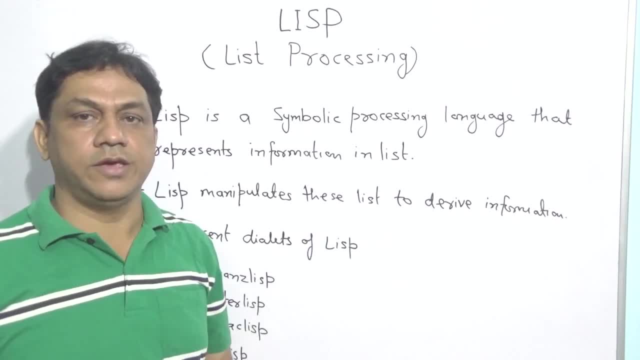 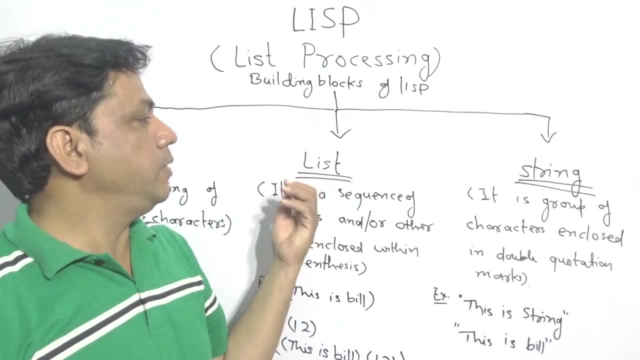 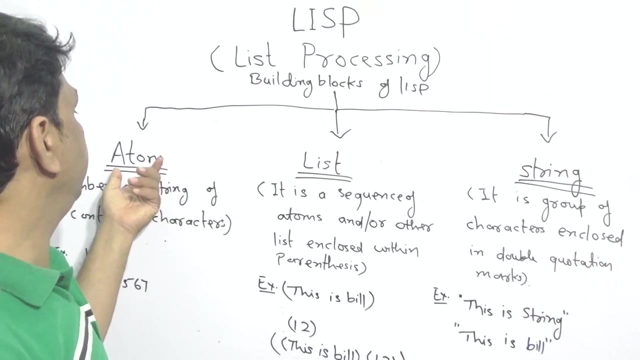 different building blocks of the list programming language. okay, now this is all about the building blocks of the list. building blocks means what are the basic blocks in which way we will write the list programming language. okay, so these are the three building blocks of the list programming. first is atom. 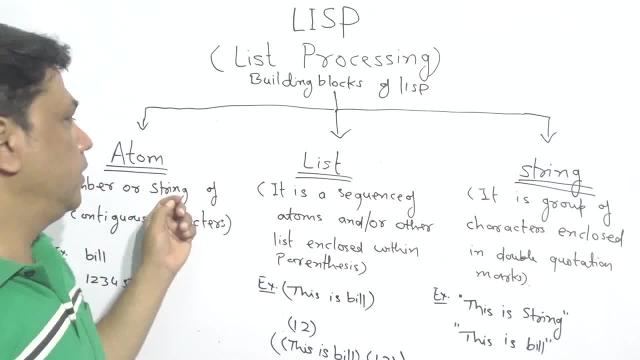 second is list and third is string. now atom is the most basic building block of the list. in atom we are writing only the number or string of. continuous character means we can write any character or any string or any number, just like this, like this example build. we are writing only the one word is here, so it become 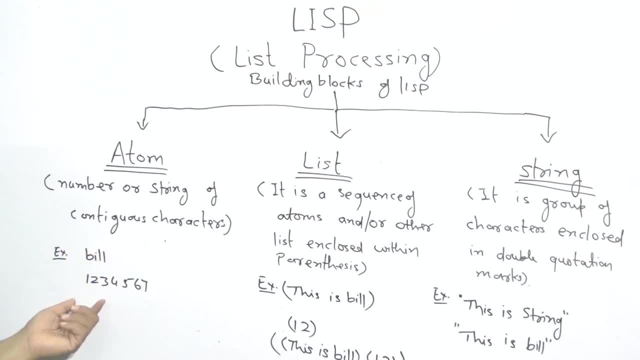 the atom. here I am writing only a number now numeric value is there: 1, 2, 3, 4, 5, 6, 7. so this is the atom. that means this is basic, lowest building block of the list. okay, so this is the atom. atom is the most basic building block of the. 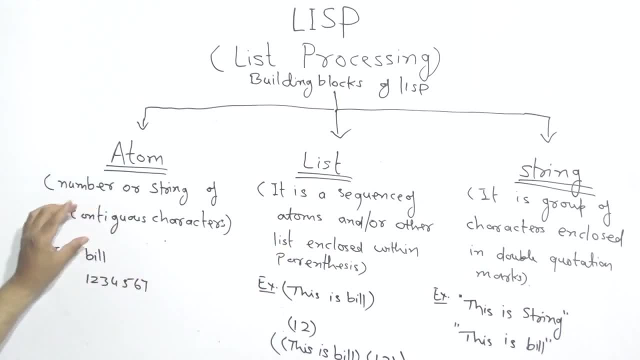 list. the second term list. list means if we are, if we enclose this atom just like a bracket here or here, or if we take the list which is enclosed by in parenthesis, then become. the list means list is the sequence of atom or other list enclosed within the parenthesis. this is our normal basic atom when we put parenthesis. 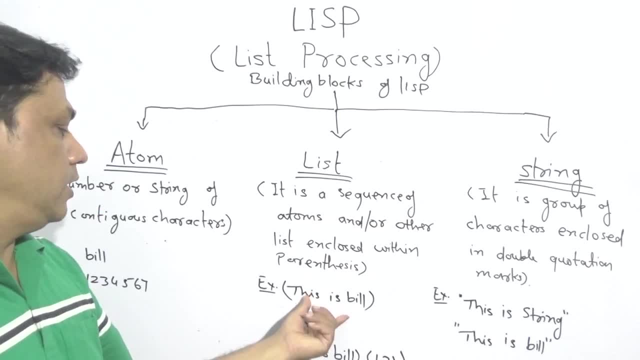 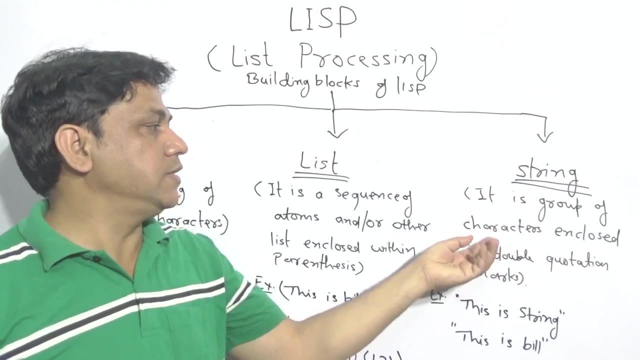 both the sides then become our list list. this is the numeric value: 1, 2, 3, 4. when I put the parenthesis here, then it becomes a list and this is already. list is there. this is the one list is there when I group. this list and category is of all about the string. string is a. 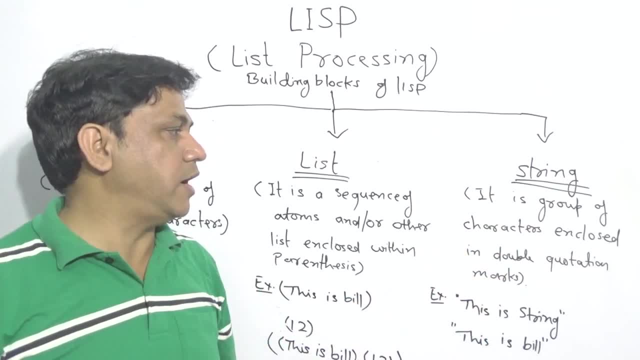 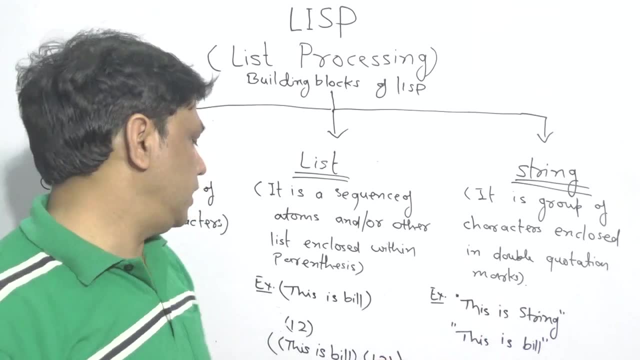 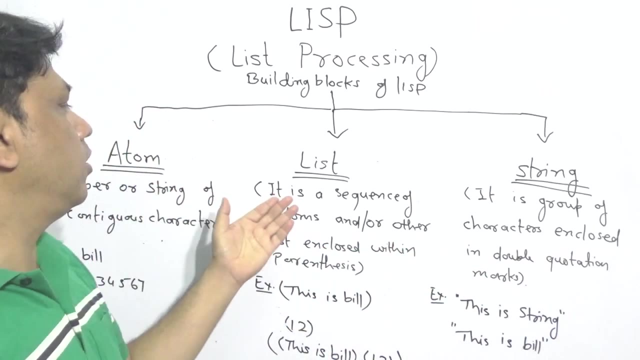 group of character enclosed in double quotation marks. me if that means if we put double quotes marks within the character, that it's become our string, just like a bill. if we put double quotes marks here then become the string string. so this is the three basic building block of the list of programming. 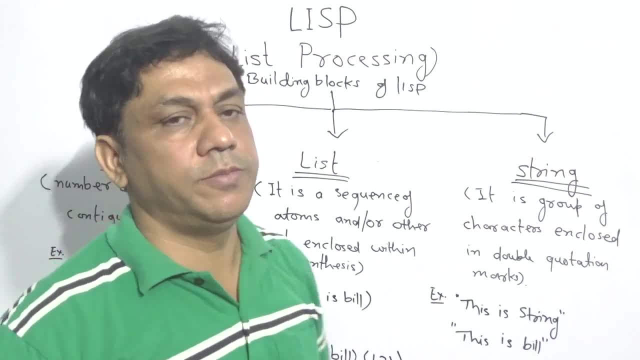 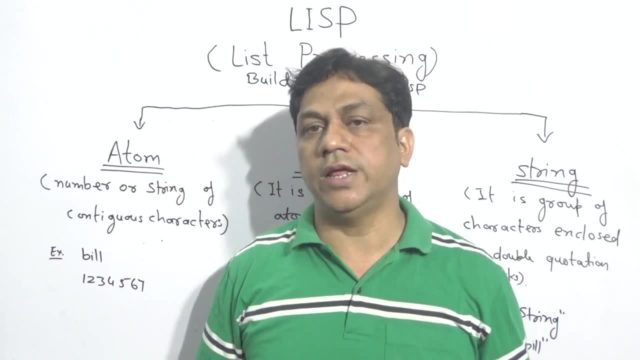 language. okay, so from the next video we will do the programming of the list here. for right now it is enough and for watching more videos like this, please subscribe my channel and share with your friends. thanks for watching.